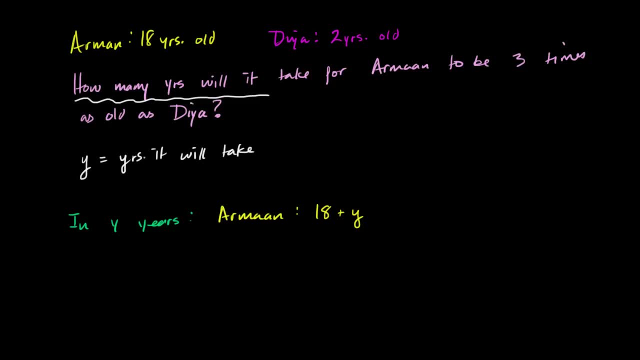 So in y years Arman is going to be 18 plus y. And what about Dia? How old will she be? How old will she be in y years? Well, she's two now, And in y years she'll just be two plus y. 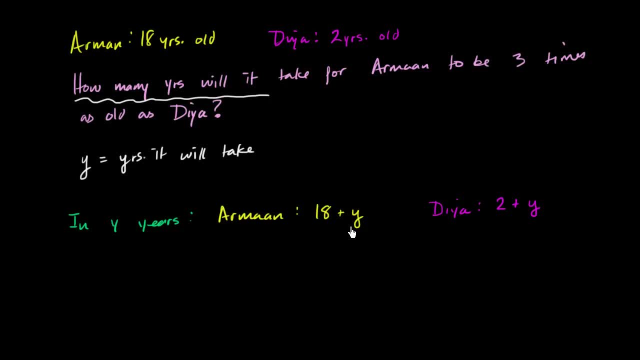 So what we're curious about, now that we know this, is how many years will it take for this quantity, for this expression, to be three times this quantity? So we're really curious. We want to solve for y, such that 18 plus y is going to be 2.. 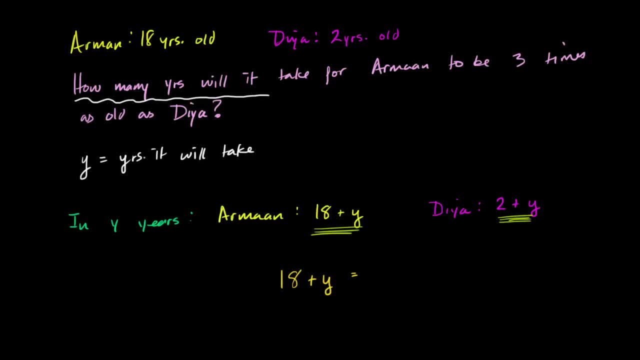 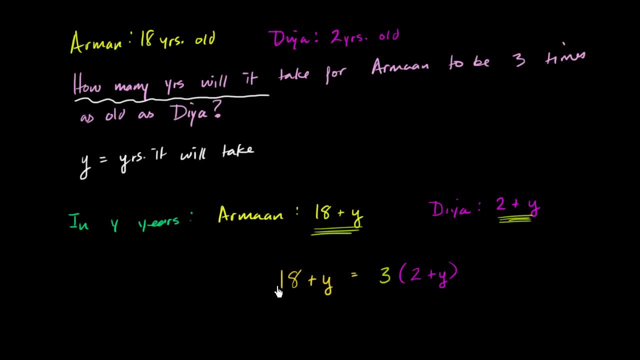 3 times 2 plus y Notice this is Arman in y years, this is Dia in y years, and we're saying that what Arman's going to be in y years is 3 times what Dia is going to be in y years. 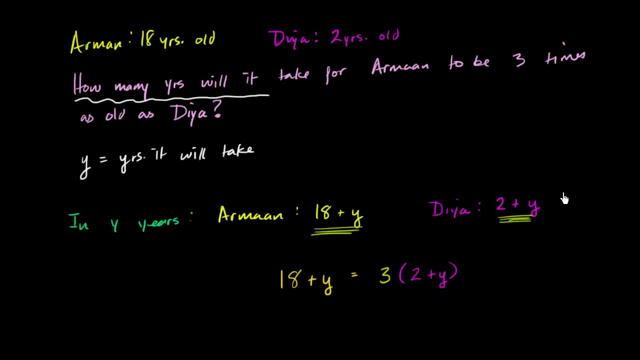 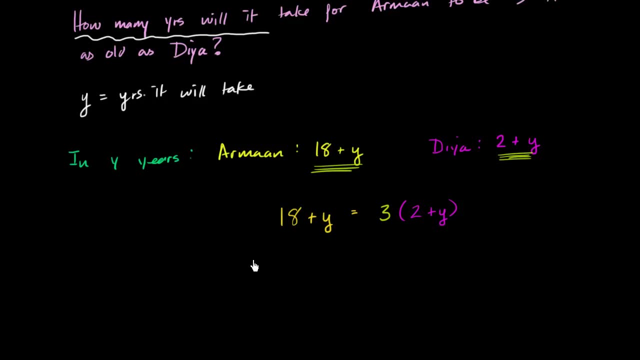 So we've set up our equation. now we can just solve it. So let's take this step by step. So on the left hand side, I'm going to put this in a new color, just so I don't have to keep switching. 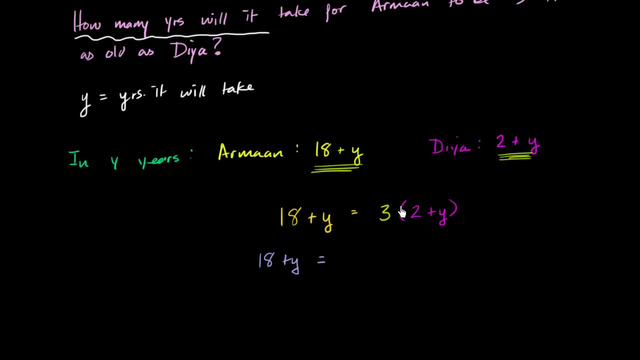 So on the left hand side I still have 18 plus y And on the right hand side I can distribute this 3.. So 3 times 2 is 6.. 3 times y is 3y, 6 plus 3y. 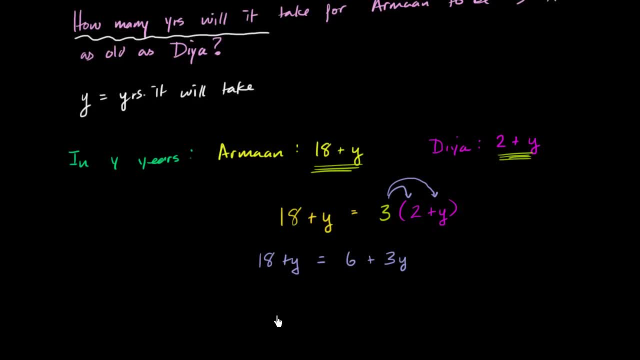 And then it's always nice to get all of our constants on one side of the equation, all of our variables on the other side of the equation. So we have a 3y over here. We have more y's on the right hand side. 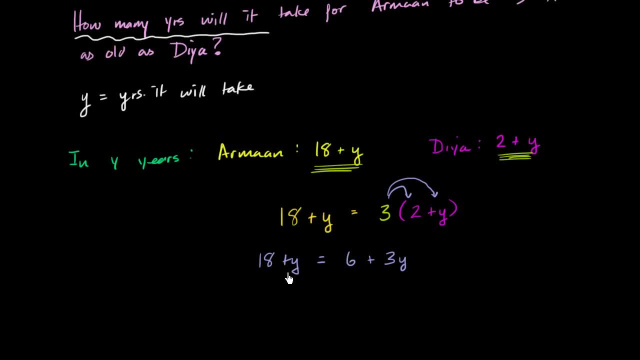 than the left hand side. So let's get rid of the y's on the left hand side. You could do it either way. you could end up with negative numbers. So let's subtract a y from each side And we are left with 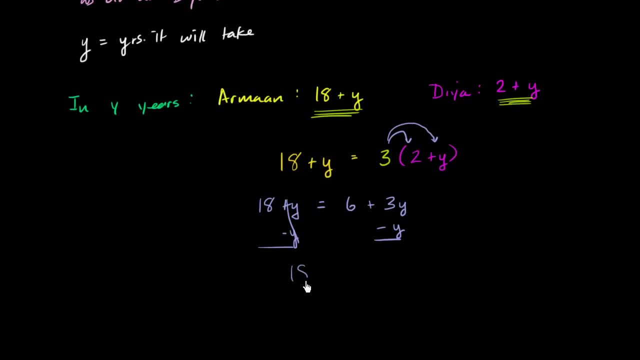 we are left with, on the left hand side, 18.. And on the right hand side you have 6 plus 3y's. Take away one of those y's, you're going to be left with 2y's. Now we can get rid of the constant term here. 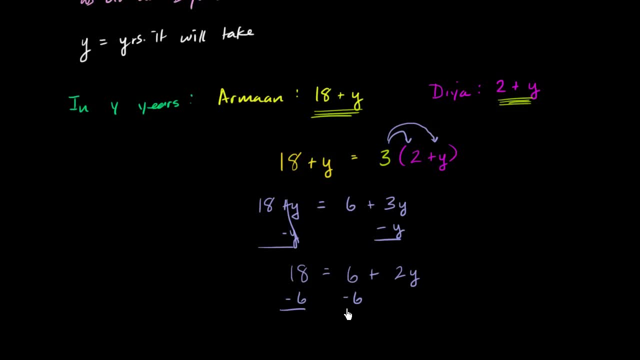 So we will subtract 6 from both sides. Subtract 6 from both sides. 6 minus 6 is 12.. The whole reason why we subtracted 6 from the right was to get rid of this. 6 minus 6 is 0..